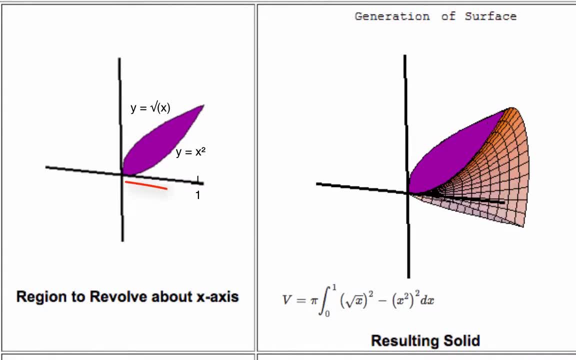 So here's another illustration of let's take the area bounded between these two regions and let's revolve it around the x-axis here and you can see that we get this as our resulting solid. 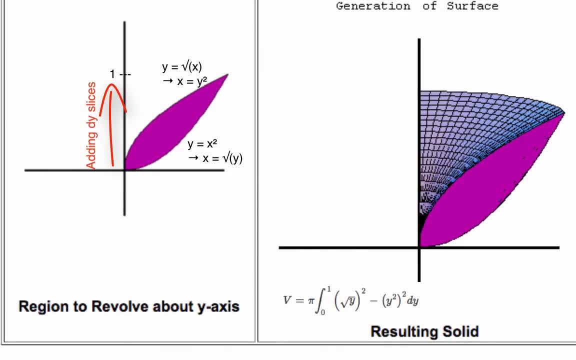 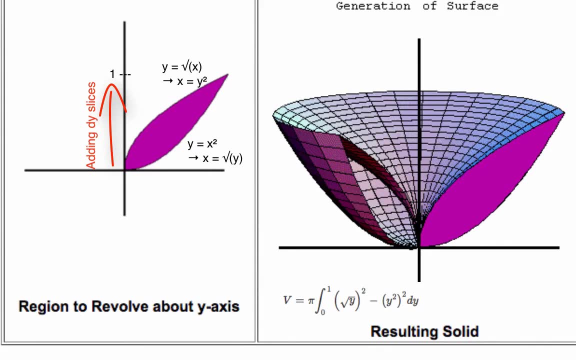 And we can take that same exact region between these two curves and revolve it around the y-axis and here is the shape that it will end up looking like. you 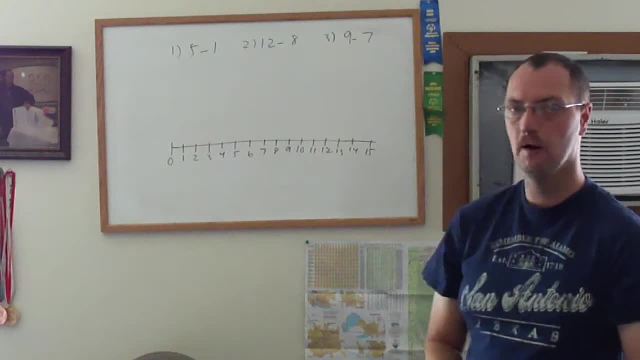 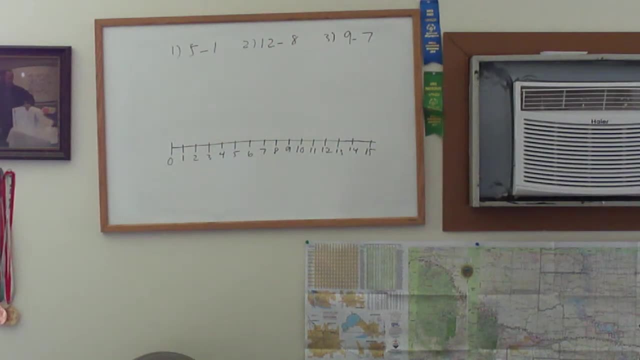 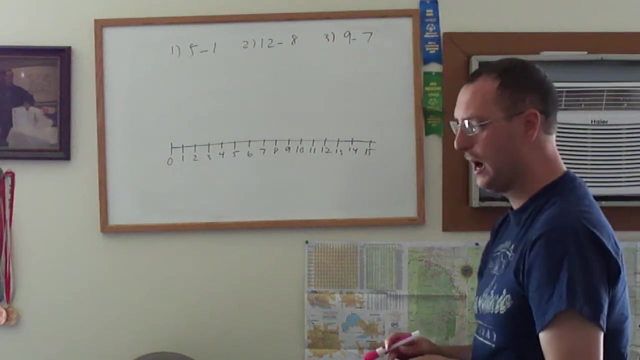 Hi, welcome to another lesson to A Replicant for a Confused. First of all, we still only have a short little quiz that we have. Today's lesson is going to subtract whole numbers. 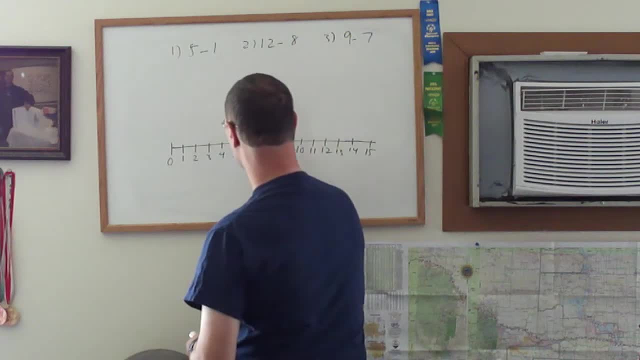 5 minus 1. This is how it is. Number 1, number 5, and we can go down 1. Which equals to 4. Alright, so, and we can use the ring this time. 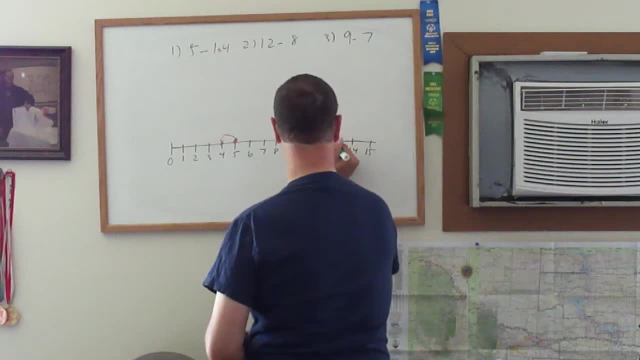 Comparison is 8. There's a 12 right there. So we have 8. 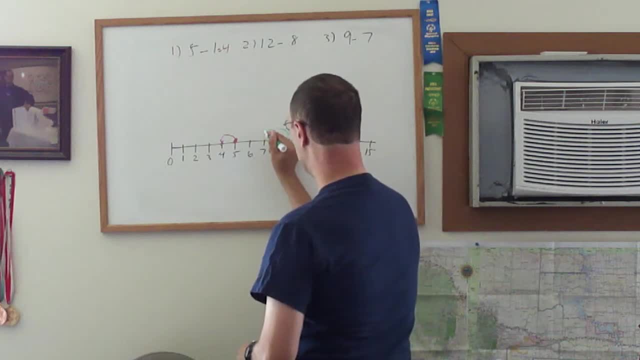 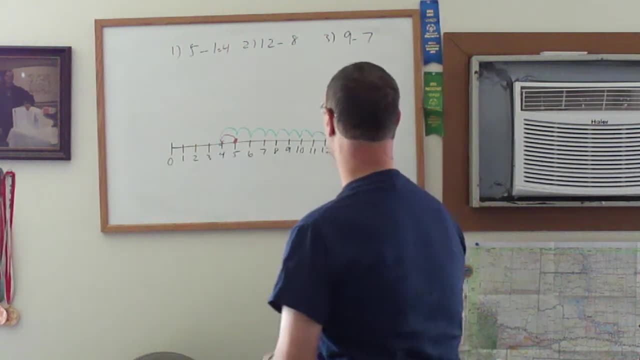 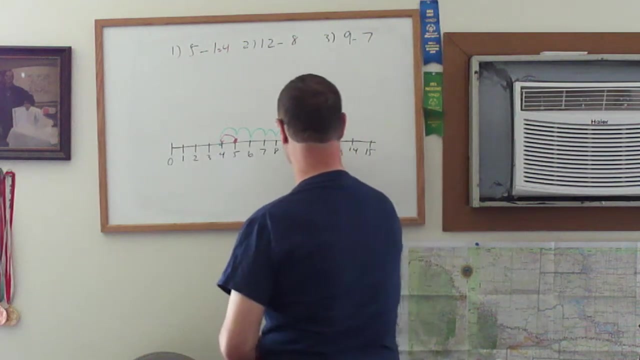 1, 2, 3, 4. 5, 6, 7, 8. Again, 4. And number 3. 9 minus 7. Right there.